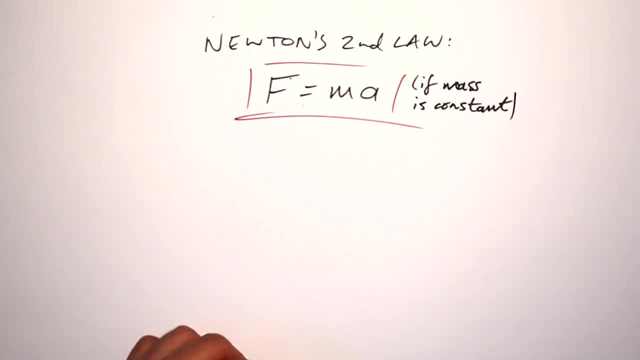 constant, Because a more general way of saying this is: if a force is exerted on an object- a resultant force that is, then its momentum changes, and momentum is made up of mass and velocity. But if mass is constant, then it's just velocity that changes. That means that we have an 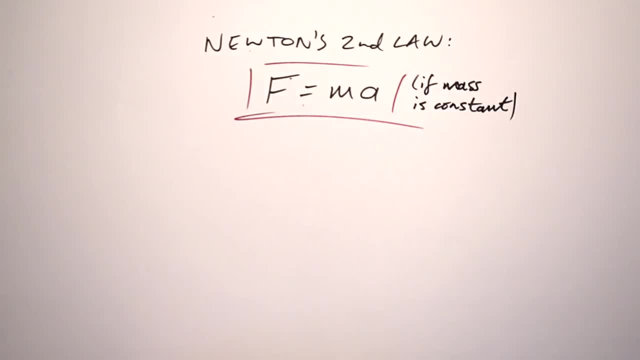 acceleration. This applies to GCSE and A-level, but we're going to start off with the easy GCSE part. By the way, if you haven't seen my easy vectors trick video, please go away and watch that first, because life is too short to draw millions of triangles for trigonometry And also it's worth. 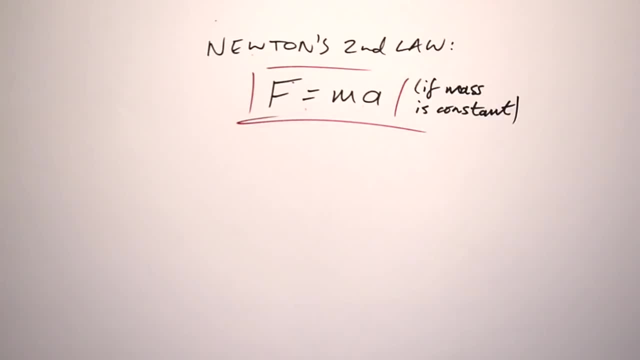 having a look at my other videos. If you haven't seen my other videos, please go and watch. that, my force and the furious video that we made with some of my pupils in science club a couple of years ago, which is a bit of fun And you can hear my amazing Vin Diesel and Paul Walker impressions. 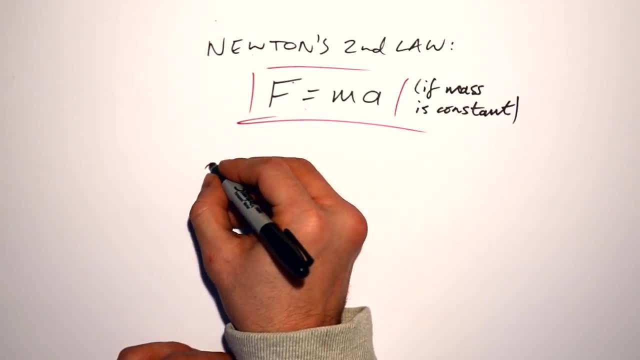 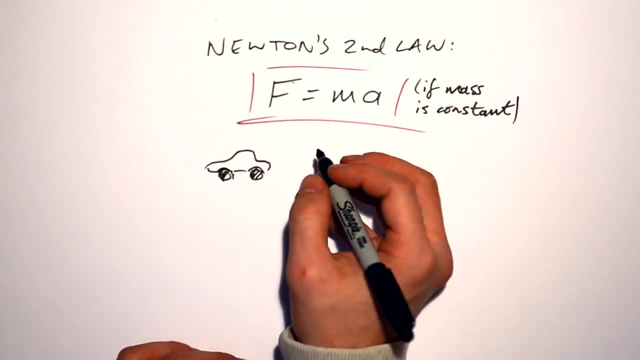 Anyway, moving on, If you have a car- and I'm going to try and draw good cars, because one guy was telling me that on another video that my cars are terrible and his teacher draws 3D cars compared to mine- I did cry myself. 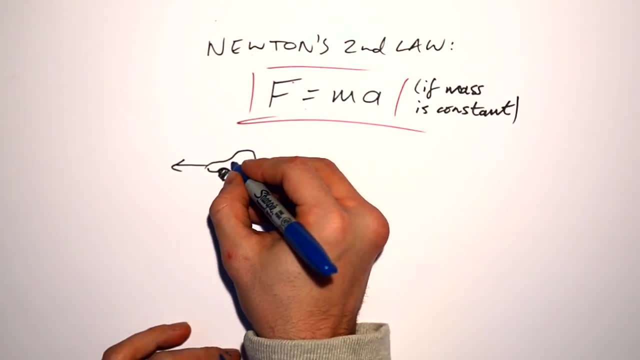 To sleep. And this car has a mass of 500 kilograms- I don't know, maybe it's a smart car or something like that- And its engine pushes forward with a force of 2000 newtons. So what do we have? We have F equals. 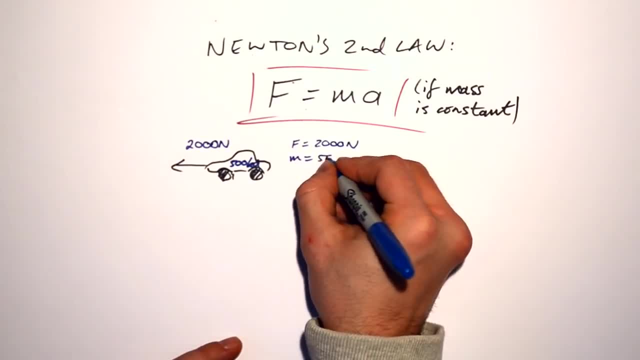 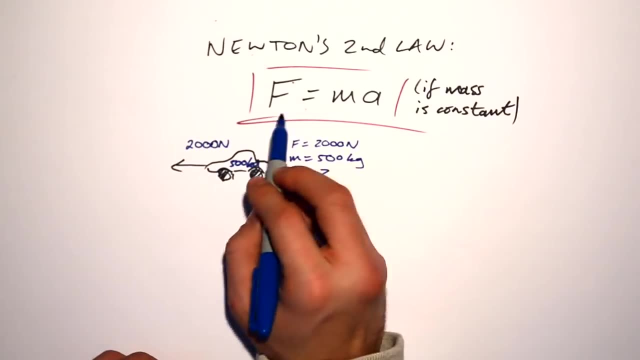 2000 newtons We have. mass is 500 kilograms. We want to find out acceleration. How do we do that? Rearrange it. You should be able to rearrange it. You should be able to rearrange this without a triangle. Hopefully you should end up with acceleration. is force divided by mass or force over? 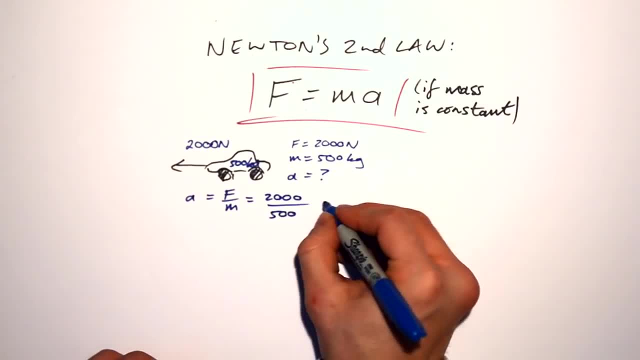 mass. So that's 2000 divided by 500 equals four meters per second squared. GCSE people, you can write it like this. You should be writing it like that. That's the air level way, That's the GCSE way of writing meter per second squared. So that's nice and easy Of. 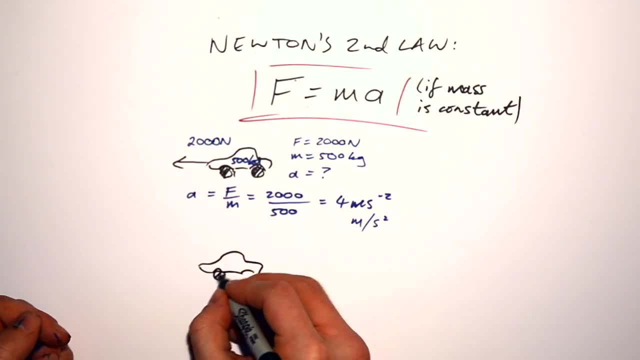 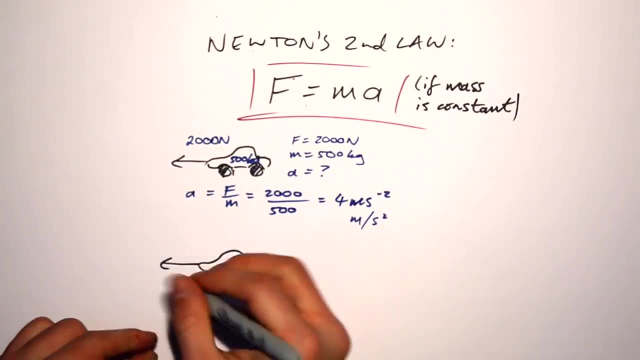 course, if there was a drag force pulling in the opposite direction, So still pushing with 2000 newtons. But the problem is is that we have a drag force. Frictional forces could be air resistance could be friction, Don't know. Still 500 kilograms. 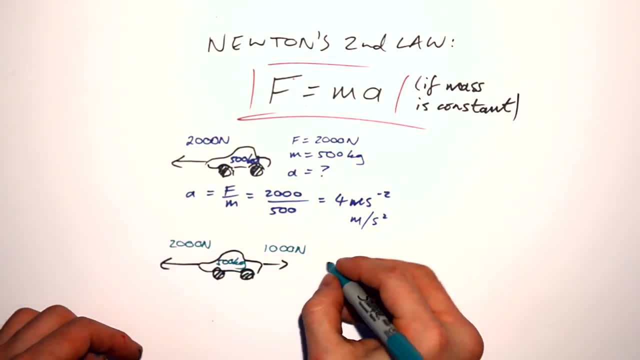 But of course that our resultant force is not going to be 2000 newtons anymore. It's going to be 1000 newtons, Because 2000 take away 1000 newtons of drag force, Give it a resultant force Of 1000 newtons. Divide that by 500 again, And that gives us a slower acceleration of two meters per second squared. 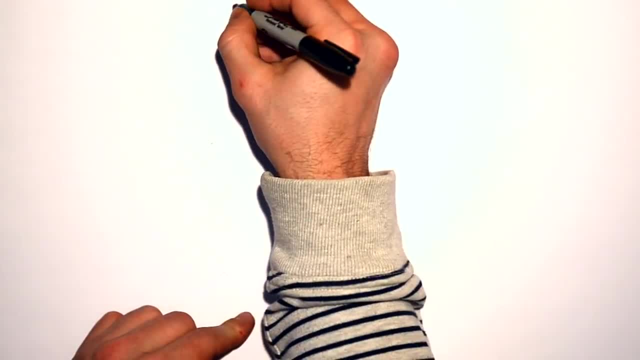 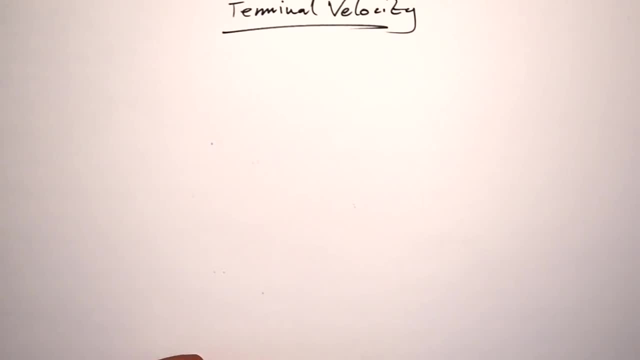 So let's talk about terminal velocity really quickly. Terminal means basically final, So we're talking about some things, final velocity. Now, this works for skydiver in particular, But it also works for Anything really that has that experiences drag forces, so it could be a car as well, but let's talk about a skydiver. 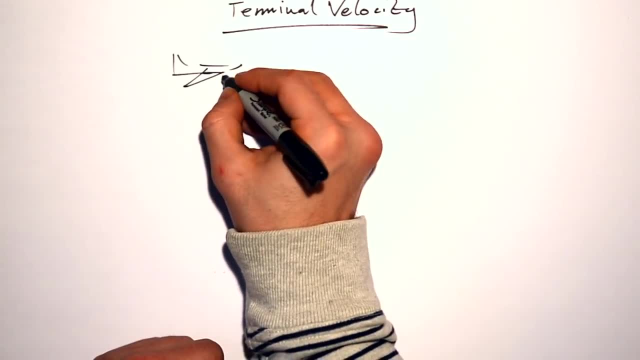 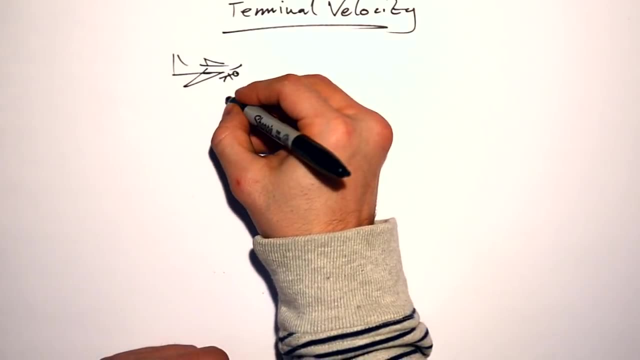 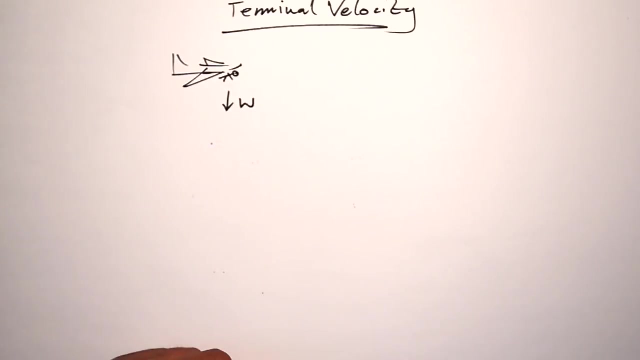 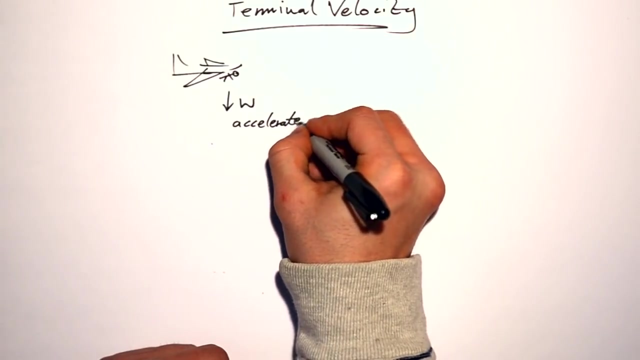 now, when a skydiver jumps out of a plane, there they are. they start falling and we have the weight pulling downwards. but there's no other force acting on them, so they start accelerating downwards big tick. but as they start falling more and more, she looks very happy. the weight? 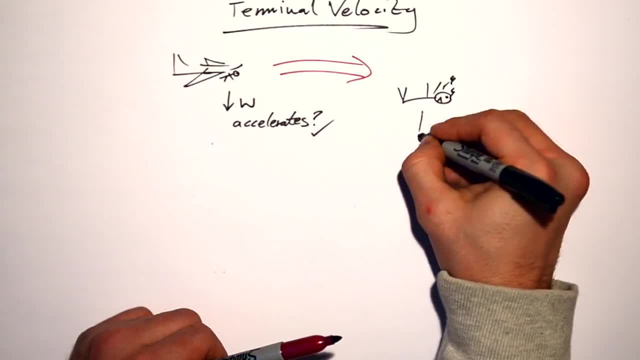 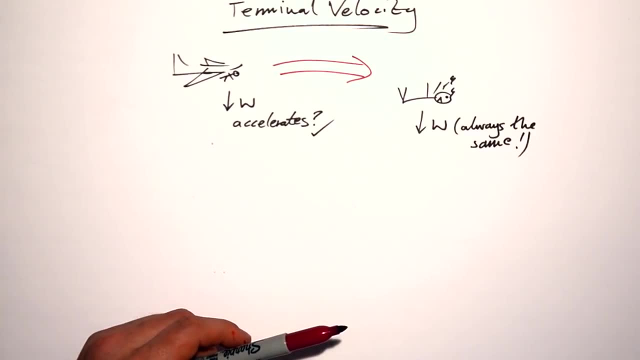 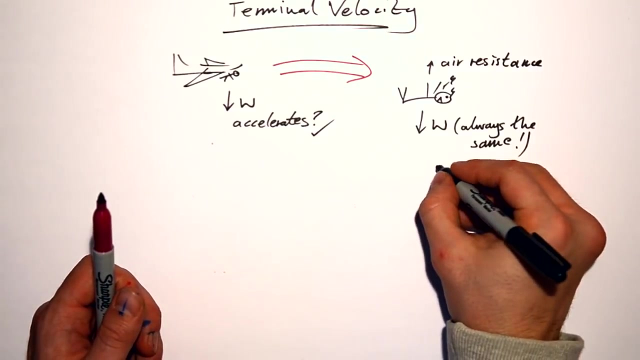 always stays the same constant, but as skydiver falls, she starts to experience a bit of air resistance, but the weight is still bigger than the air resistance, so accelerates big tick. eventually, though, skydivers are able to do a lot of things. they're able to do a lot of. 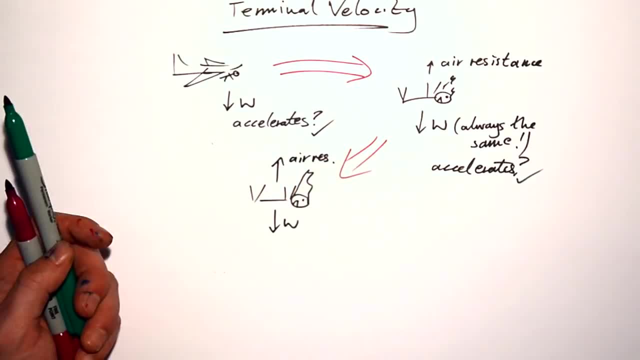 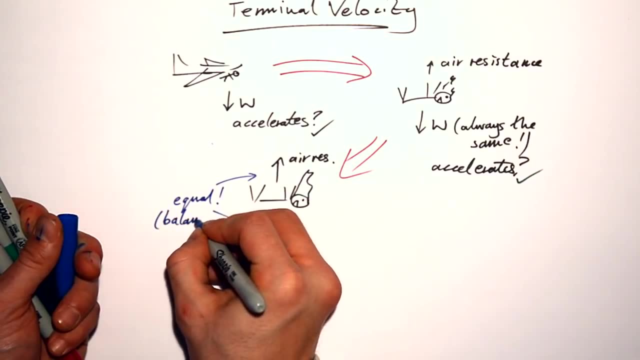 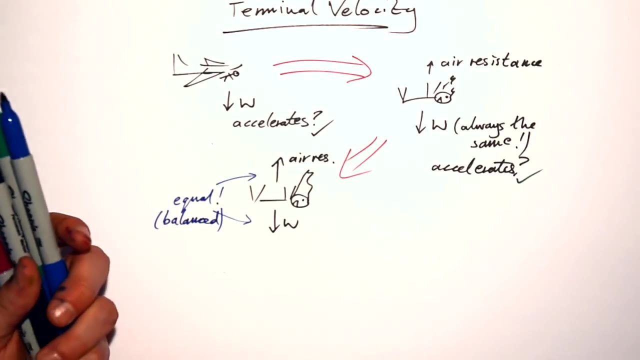 the air resistance as she gets faster and faster, they will actually equal. so we say they're balanced. that's when we wander from newton's second law territory into newton's first law territory. now we have no resultant force, there's no net force. the air resistance is as big as the weight in the opposite direction, so therefore accelerates. 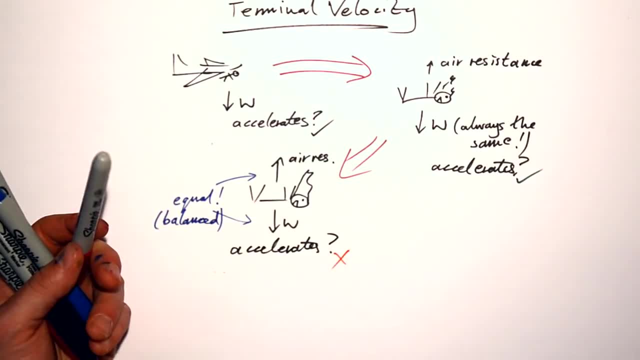 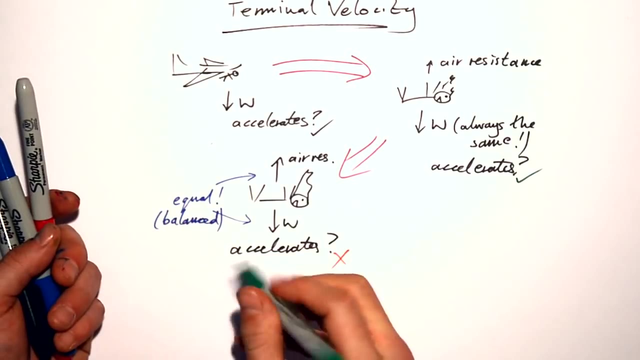 big fat. no, that does not mean that she stops. that just means that the speed that she was going, the velocity she was going at the point where this happens, that's the velocity that she keeps on going with, so she reaches terminal velocity. of course it's one last bit as well. 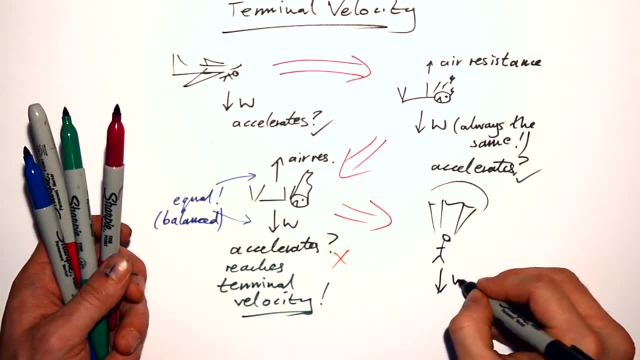 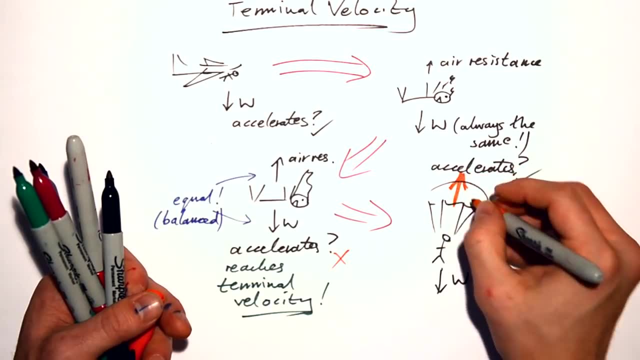 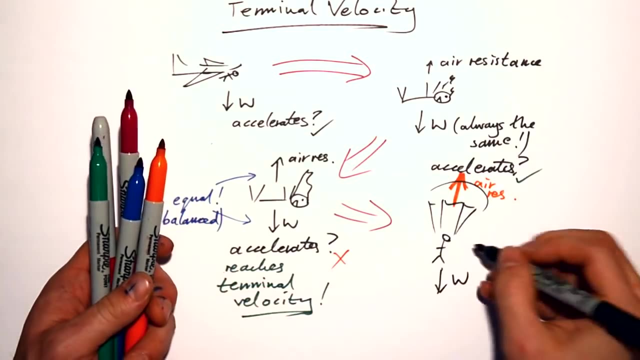 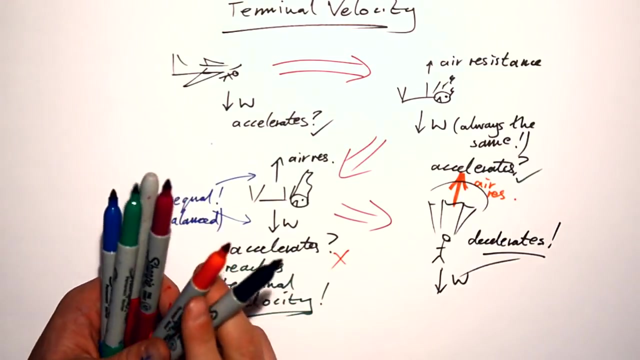 when she opens a parachute, weight is still the same, but air resistance is now massive. so if air resistance is bigger than the weight pulling downwards, she's actually going to decelerate. that means she's going to slow down. is she going to carry on slowing down? no, because eventually the 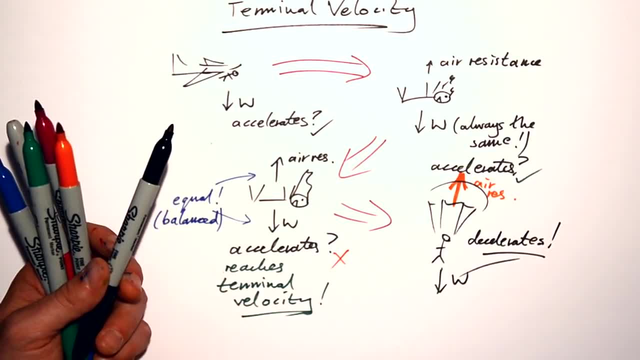 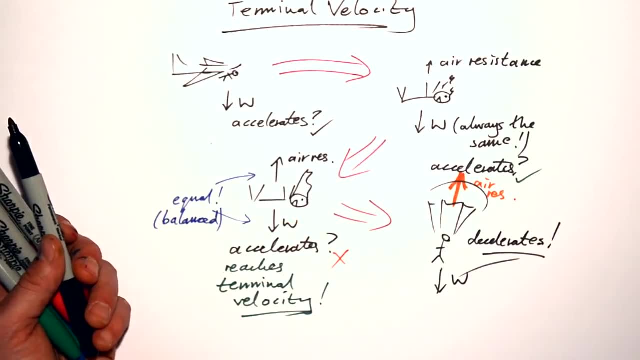 air resistance will decrease to the point where it's the same as the weight again and, no surprises- she falls at a new terminal velocity. it's going to be slower than the terminal velocity that she had here, but it's still a constant velocity. let's go with inclined plane. 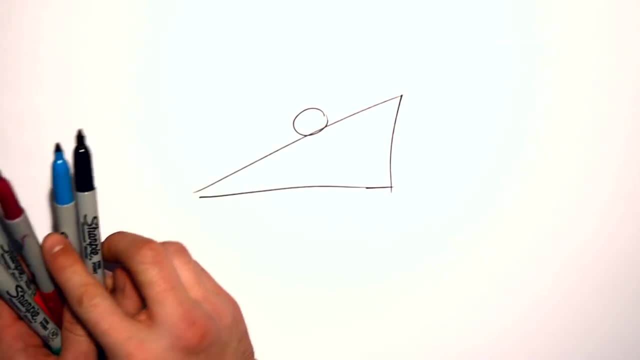 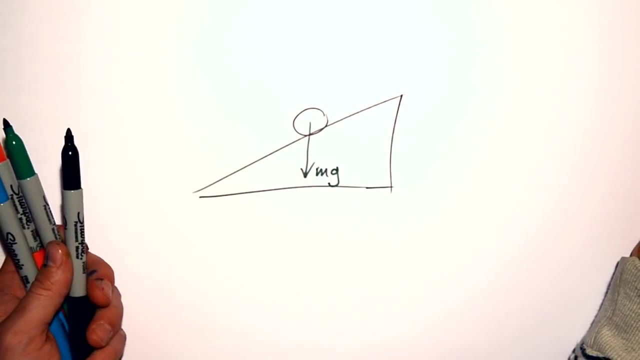 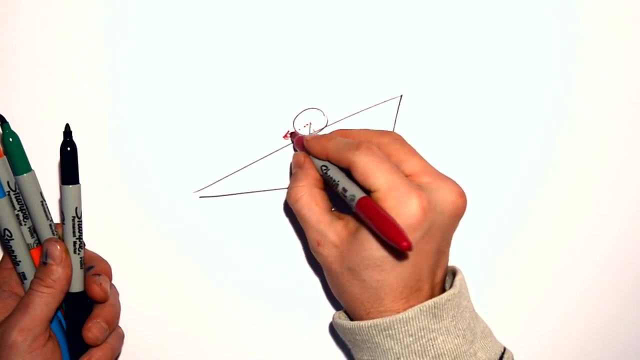 and let's say that we have a ball on here and it's free to roll down the hill. now we know that its weight is pulling downwards- and if you haven't seen my easy vectors trick video, go and see that, because this explains where i get these from- and we know that the ball isn't going to accelerate. 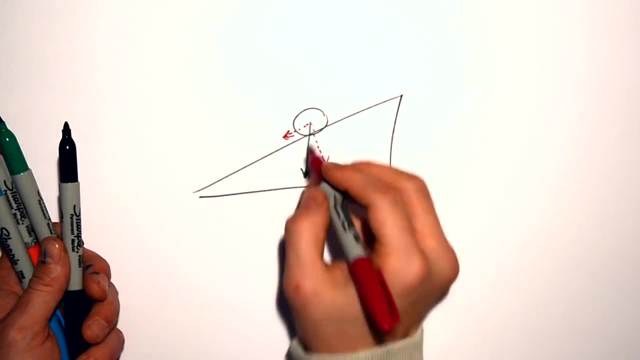 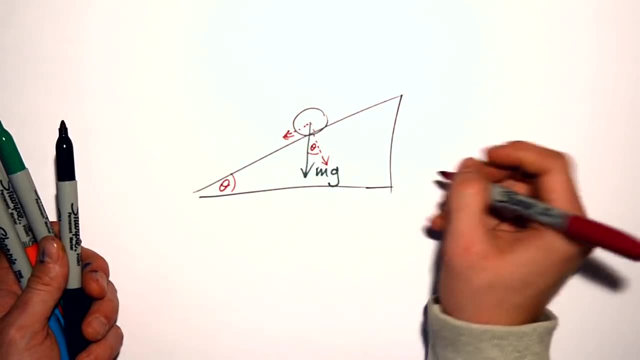 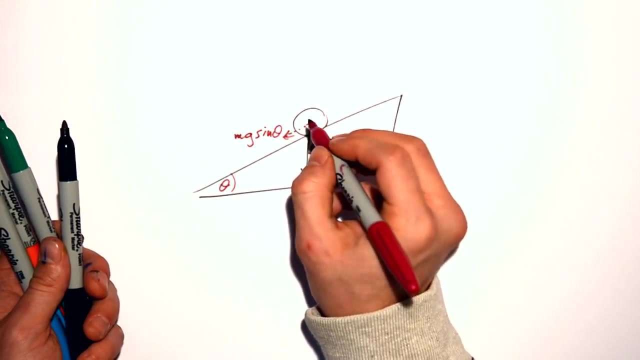 into the ramp. it's not going to accelerate this way. it's only going to accelerate this way. and if this angle here is this angle, here is theta, this angle here is also theta, turning through the angle, this is going to be mg cos theta, this is going to be mg sine theta. so i cannot say that f. 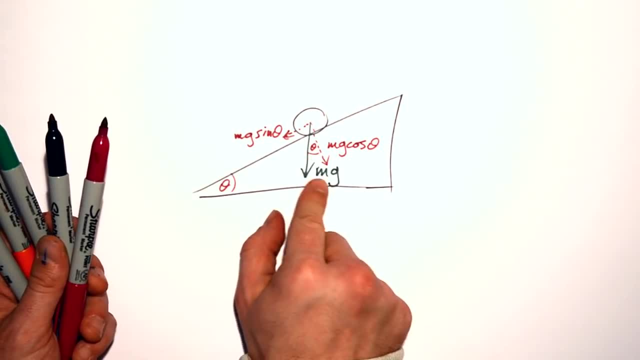 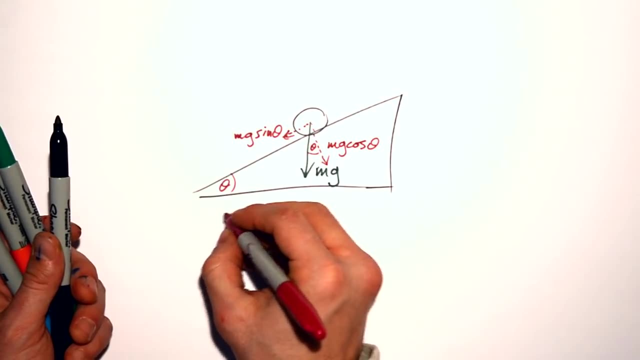 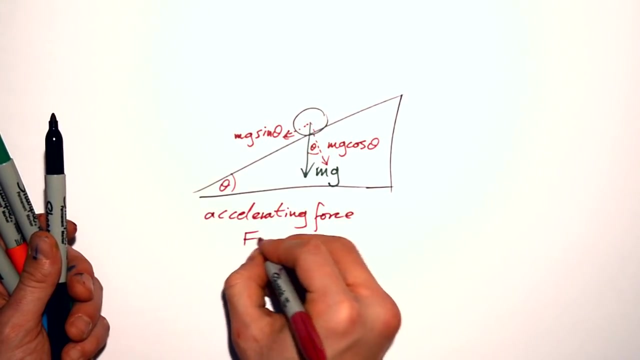 equals mg because, well, the force is mg, but the acceleration isn't going to be g because it's not accelerating this way. but i can say the accelerating force, which is what m, a always is, is going to be equals to mg sine theta. now you may notice that the acceleration, therefore, 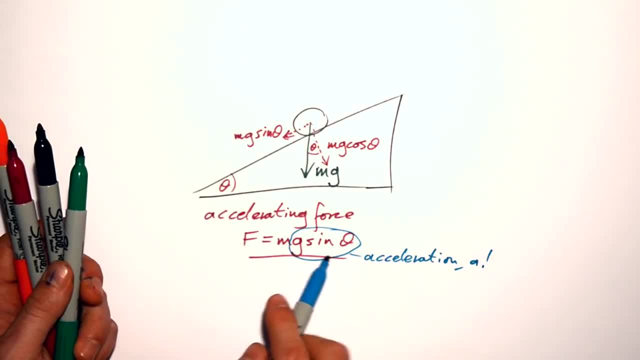 g sine theta f equals mg. sine theta f equals ma. so that means the acceleration is going to be g sine theta. that makes sense, doesn't it? because if the ball is allowed to fall under gravity, the acceleration is going to be g, but because it's only having some of that acceleration. 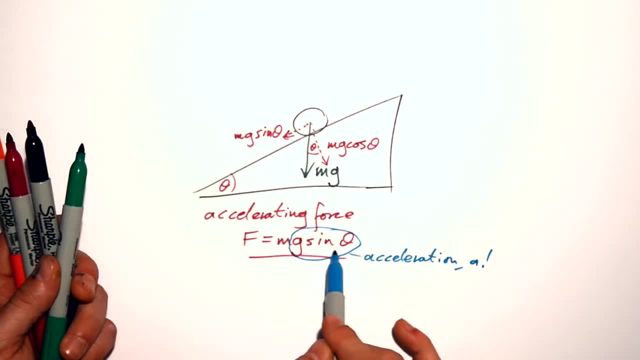 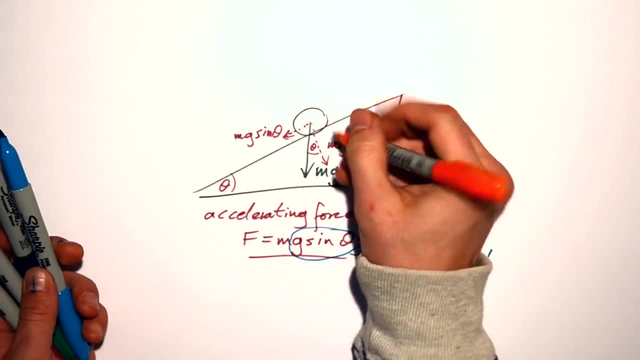 as it's accelerating down the slope, then it's going to be g sine theta worth of that 9.8 meters per second squared. we can have frictional forces pulling in the opposite direction, though it's called the fr if the ball was moving at a constant speed. 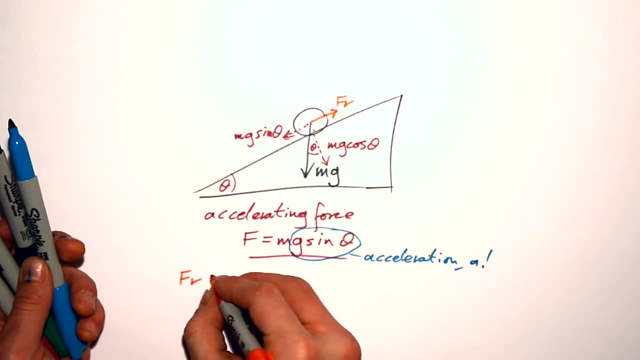 so i could say that fr equals mg sine theta, plus only if no acceleration. notice that i didn't say. if it's not moving, it is going to be true if it's not moving, but it also could be falling at a constant speed. if that is the case, 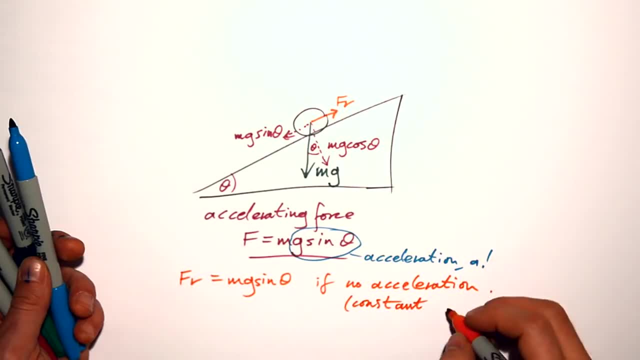 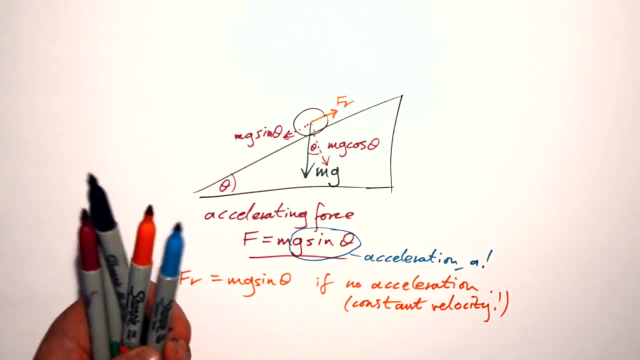 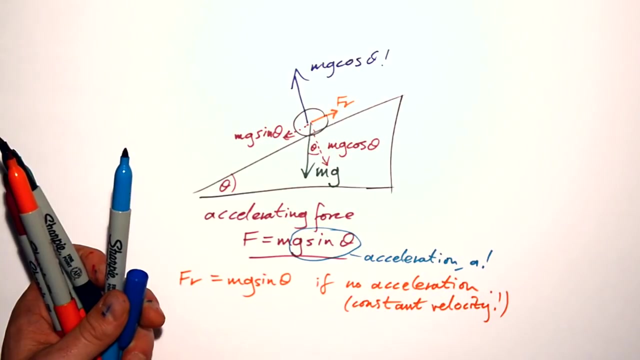 if it's not moving, then it's going to be true. if it's not moving, the frictional forces are going to be equals to mg sine theta. there's one more thing i know about this situation, and that is this: this is also going to be mg cos theta going perpendicular to the plane out of the ramp. 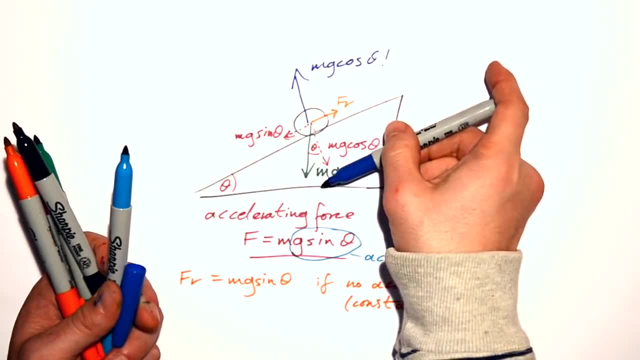 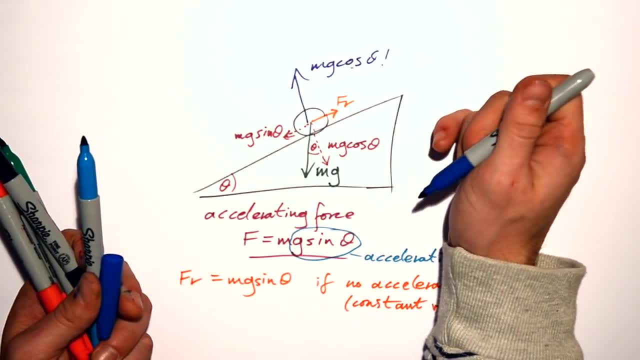 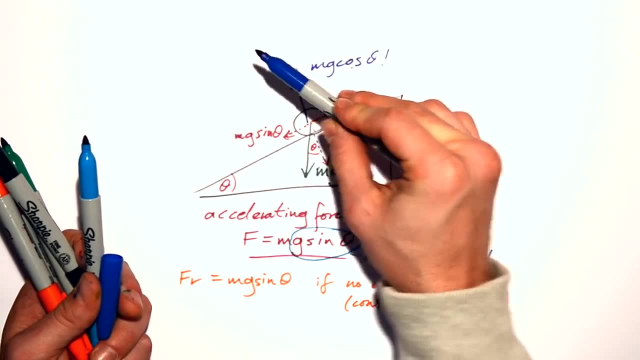 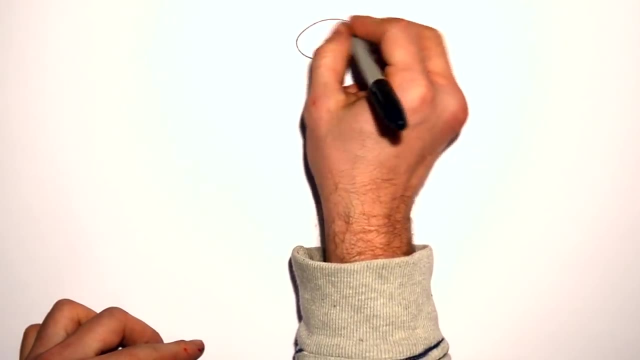 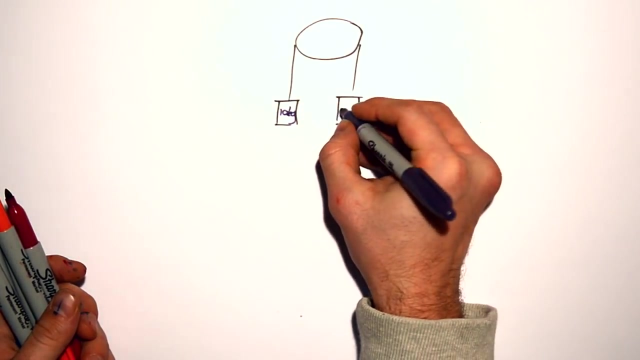